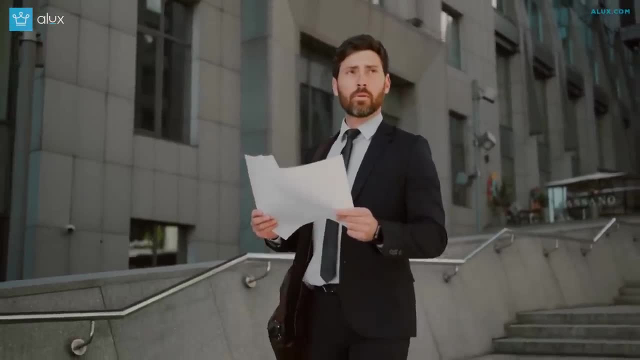 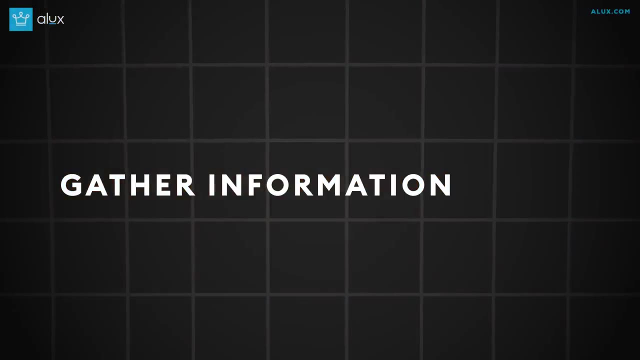 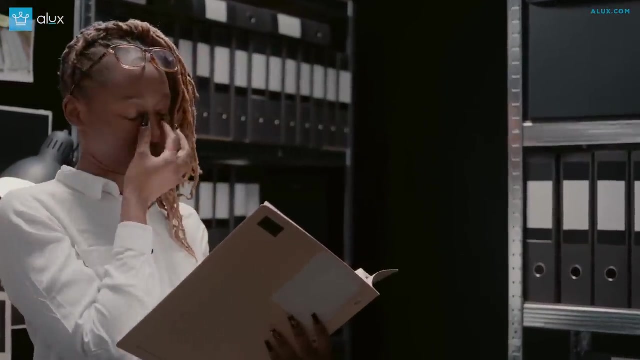 and thus ultimately overcome that challenge with efficacy and finesse. Next up: gather information. While trying to solve a problem, you practically aim to find a solution, And information is what serves as the thread that weaves together that coherent solution. 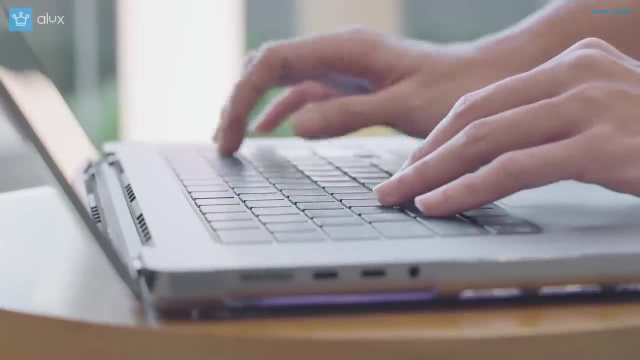 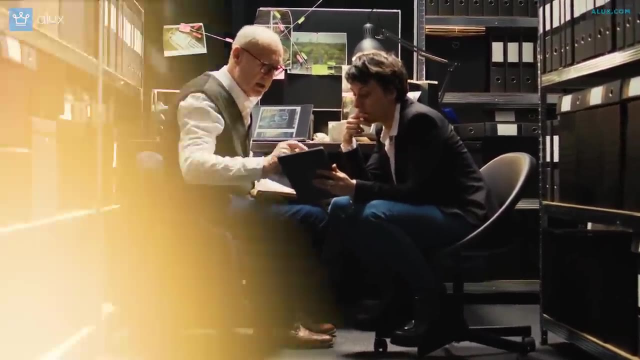 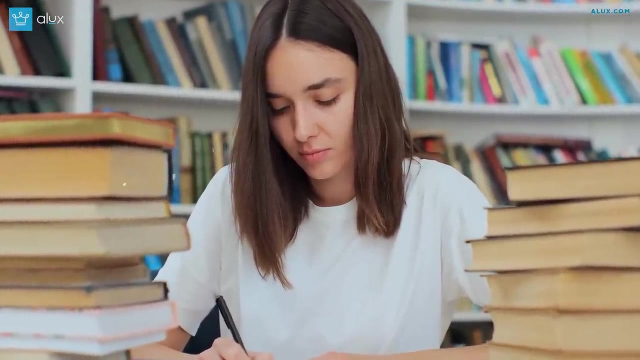 Gathering pertinent information is similar to arming yourself with a potent arsenal of insights, a reservoir from which creative and pragmatic solutions can spring up. The value of being well-informed cannot be overstated. The depth and breadth of your insights directly correlate to the level of your knowledge and the level of your experience. 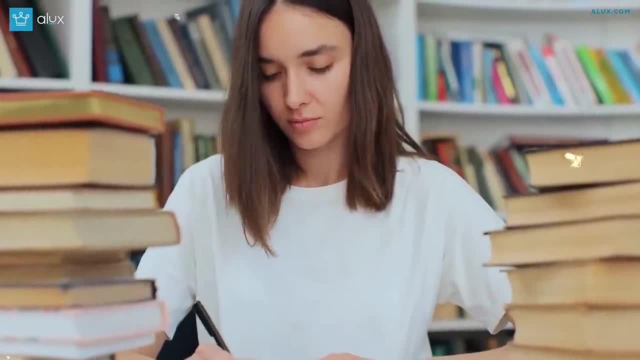 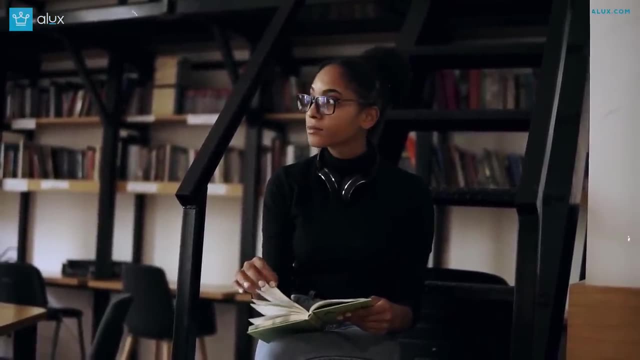 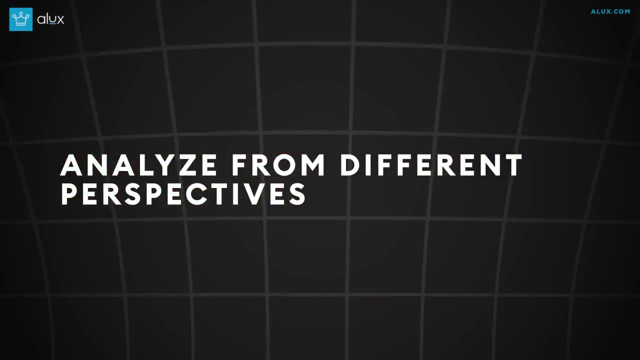 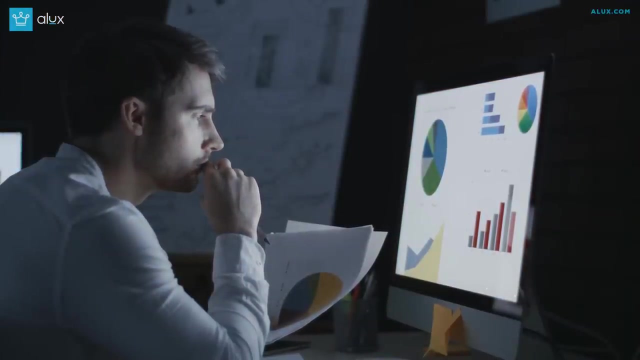 You are poised to innovate, devise ingenious strategies and navigate the intricacies of the problem space with finesse. ANALYZE FROM DIFFERENT PERSPECTIVES. In the realm of problem-solving, adopting multiple perspectives is like seeing a puzzle from various angles. Each viewpoint offers a unique piece of insight. 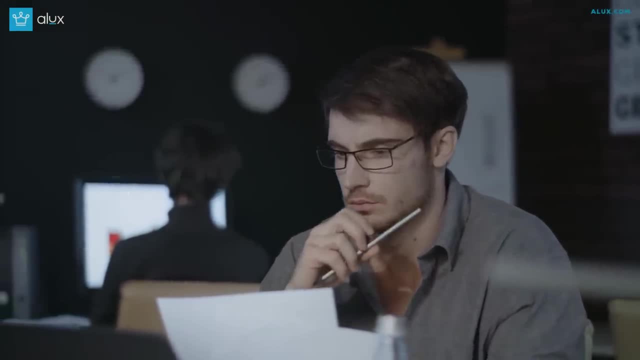 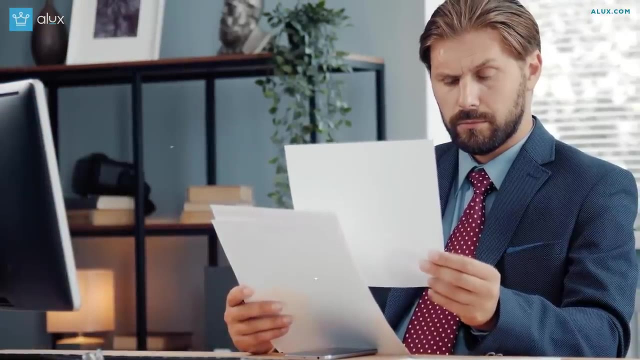 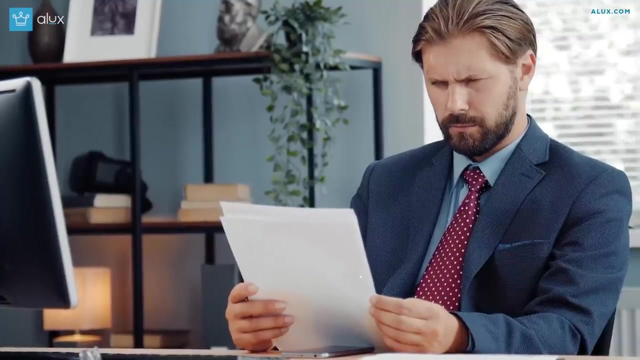 contributing to a complete understanding of the challenge at hand, Much like an artist stepping back to see their canvas in different lights. considering a problem from diverse angles unveils hidden facets and novel opportunities. This approach encourages flexibility and empathy, hallmarks of effective problem solving. By exploring a problem's dimensions from different points of view, you can identify connections, foresee potential obstacles and uncover unconventional solutions. This cognitive flexibility enhances your ability to tackle complex issues with creativity and depth. Then it's time to brainstorm. Unlock the gates of innovation with a potent problem-solving tool. 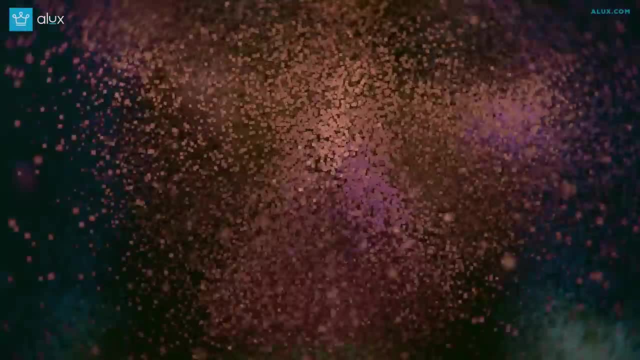 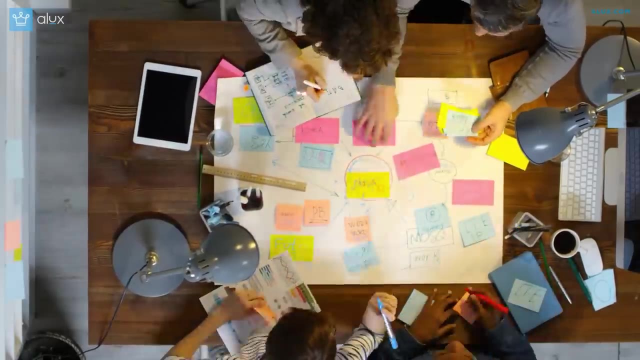 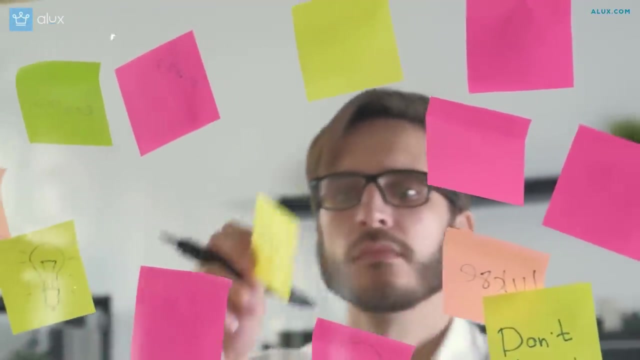 Brainstorming. And if you're wondering, yes, you can brainstorm by yourself. It's called individual brainstorming and it can do wonders. In brainstorming, the magic lies in suspending judgment and embracing the boundless realm of ideas. This liberty nurtures a steady flow of thoughts. 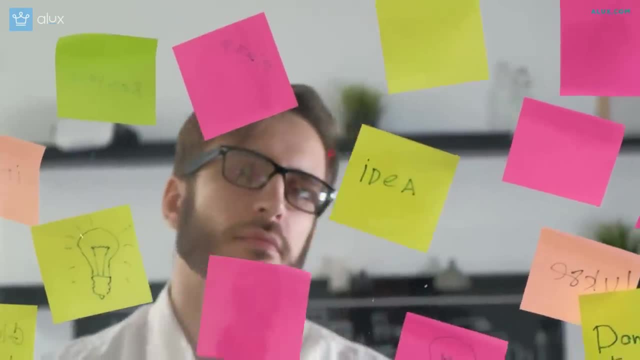 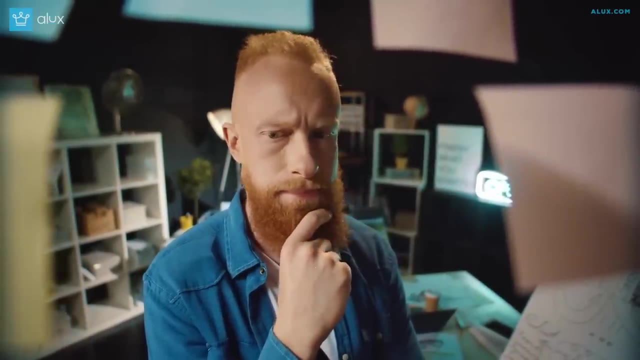 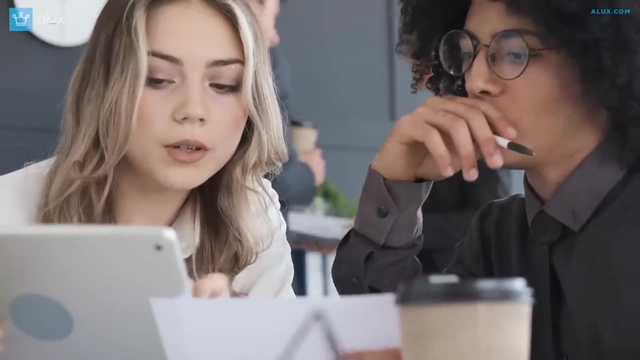 creating a fertile ground for novel concepts to sprout and flourish. Imagine this process like a pot bubbling over with possibilities. Encouraging uninhibited expression, even of unconventional ideas, cultivates the potential for groundbreaking breakthroughs. In essence, brainstorming is propelling problem-solving to new heights. 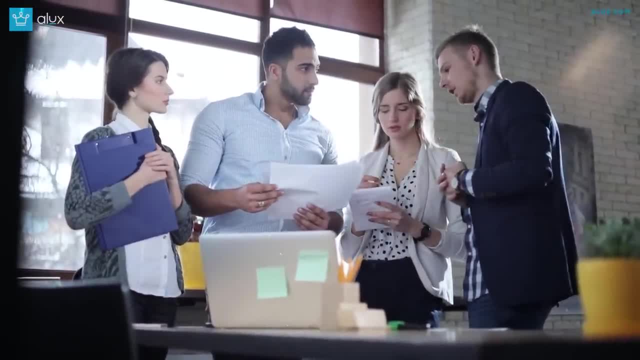 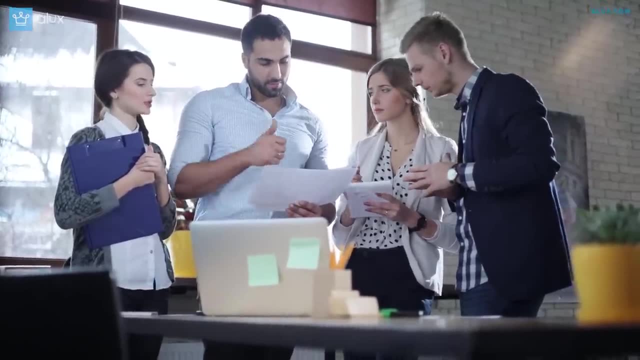 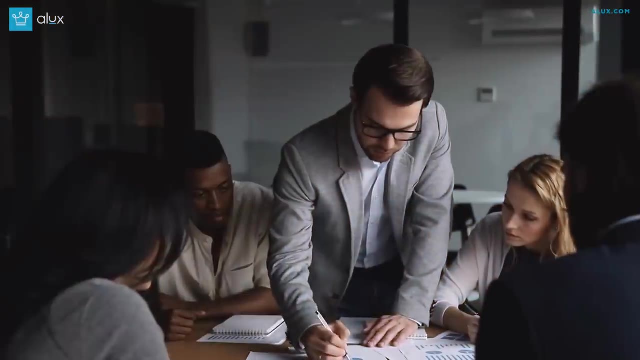 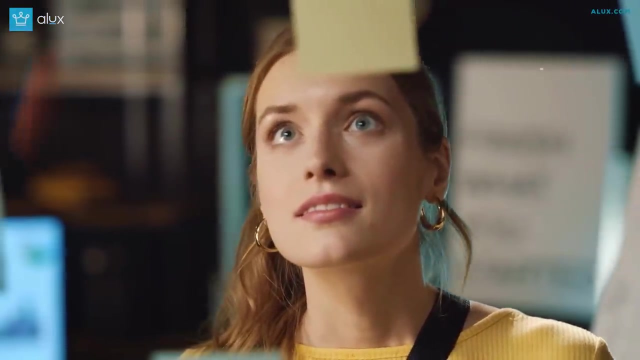 By embracing this process and fostering an environment of imaginative liberty, you can carve out a path toward ingenious solutions, thus gaining a new power. Prioritize solutions. After compiling a roster of potential solutions, the next crucial step is to methodically prioritize them. This selection process is founded upon several pivotal criteria. 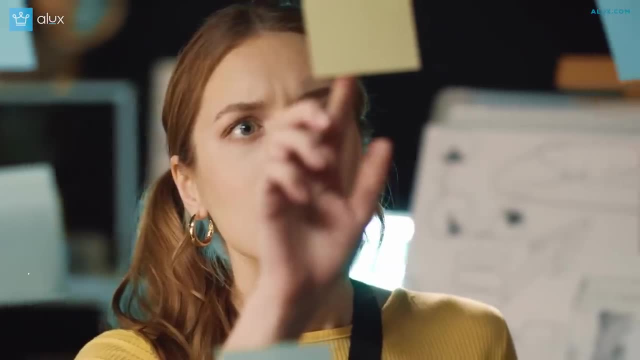 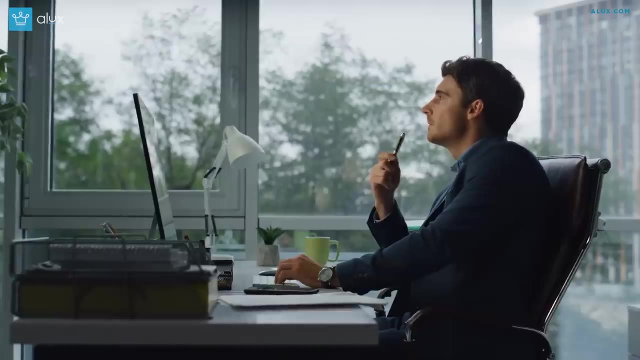 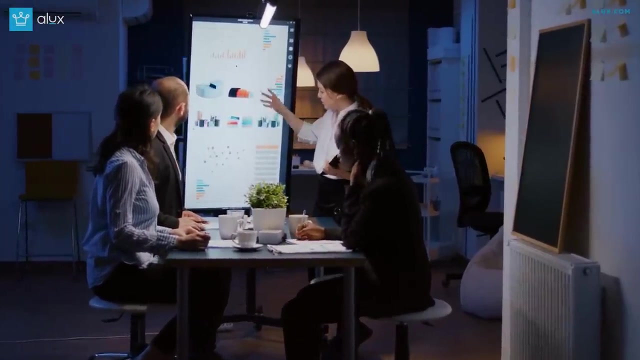 feasibility, potential impact and alignment with your objectives. By meticulously evaluating and ranking them, you can channel your energy toward those with the highest potential. This strategic approach optimizes your resources, enhances your problem-solving efficiency and facilitates the achievement of your desired outcomes. 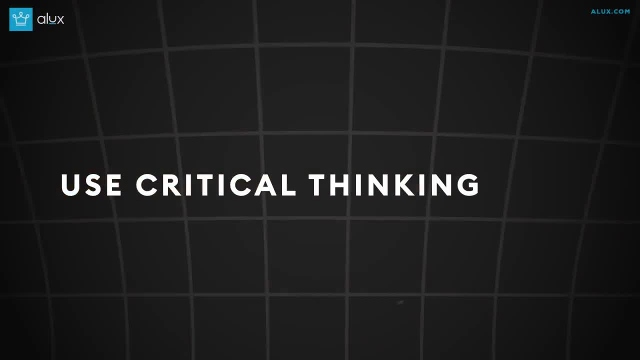 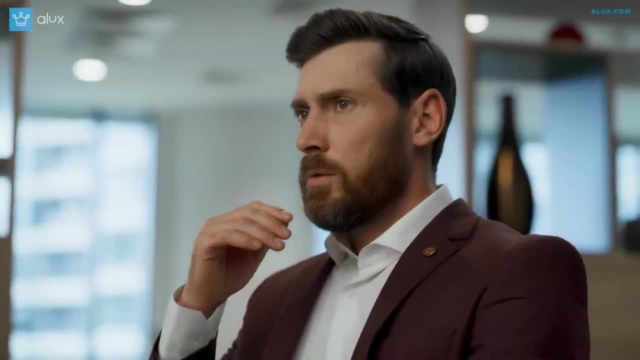 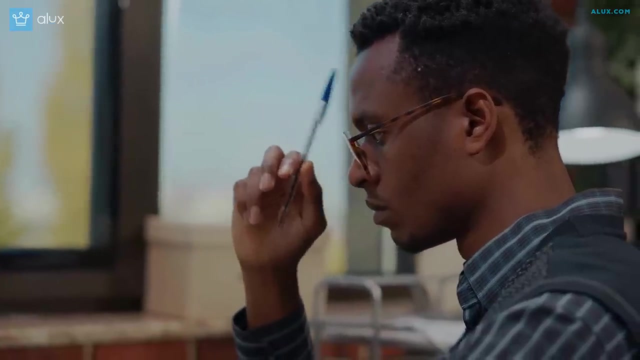 Use critical thinking. Embrace the power of critical thinking as you embark on the journey of solution evaluation. This cornerstone of effective problem-solving demands a meticulous dissection of the task of solving problems. 3. section of each potential remedy. Moreover, take into consideration risk assessment. 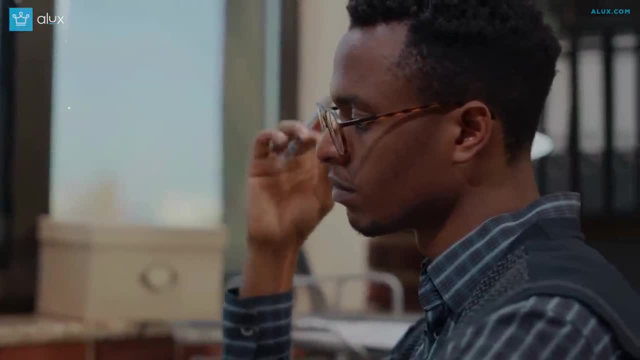 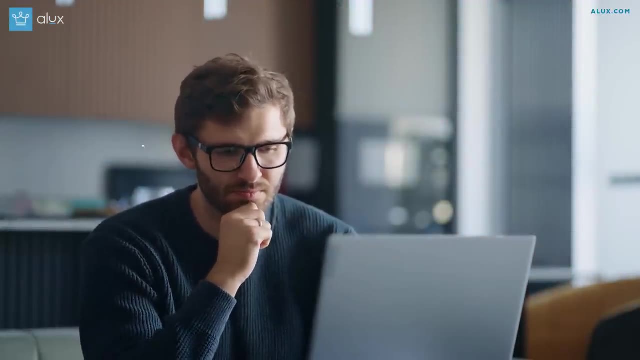 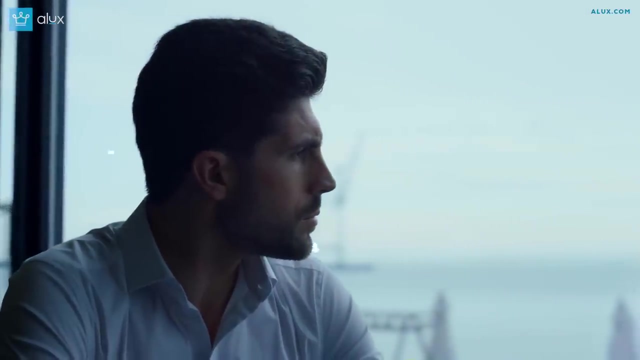 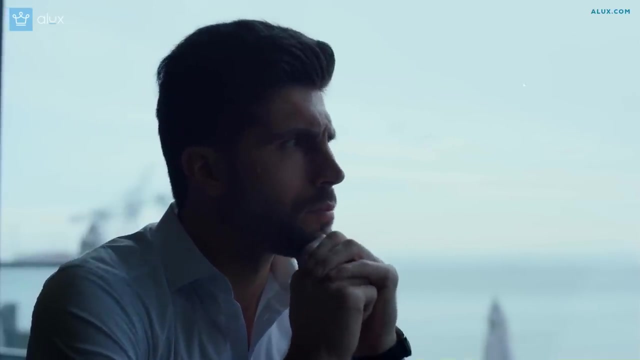 Envision the potential pitfalls and challenges that might arise during the execution of each solution. A thoughtful consideration of possible setbacks empowers you to devise preemptive strategies to mitigate them effectively. Incorporating critical thinking into your assessment process ensures that your chosen solutions are not only well-informed, but also poised for success. 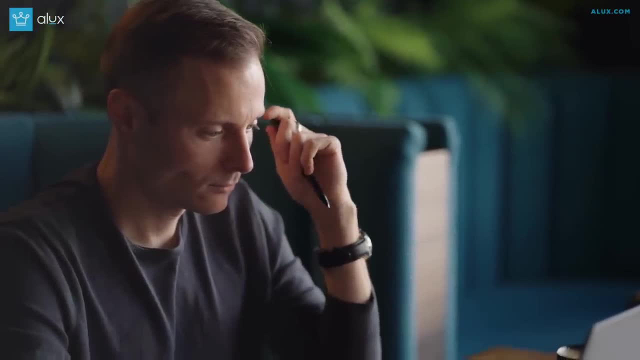 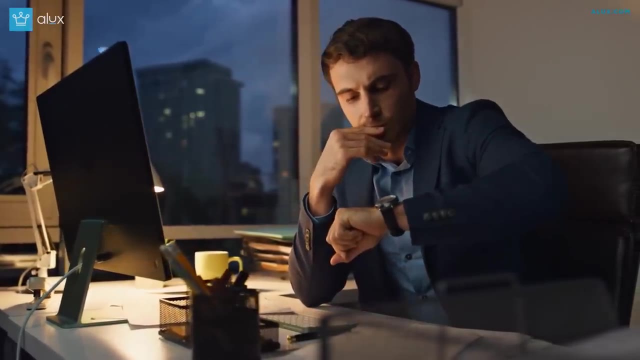 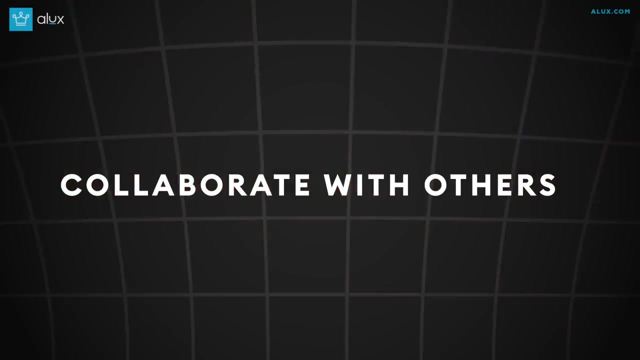 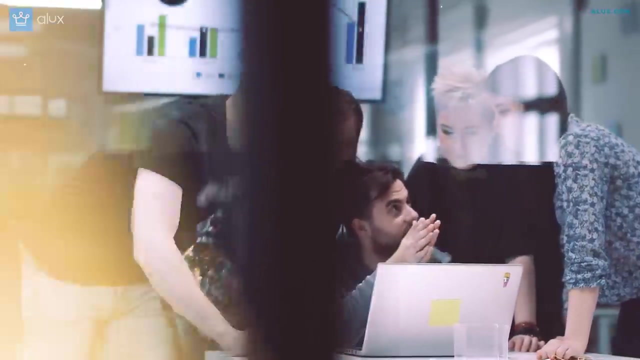 By meticulously examining pros, cons, risks and unintended consequences, you solidify your foundation for effective decision-making and propel your problem-solving journey toward comprehensive and impactful solutions. Collaborate with others: Harness the power of collaboration by engaging others in the process of problem-solving. 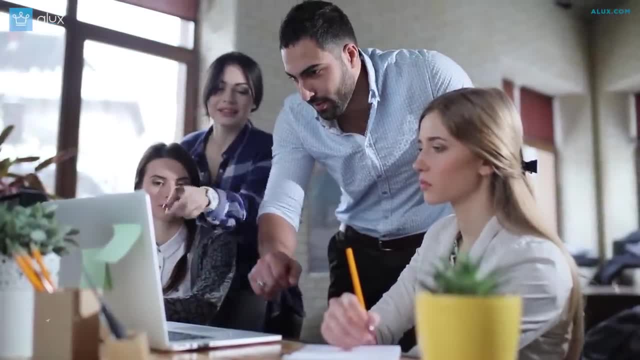 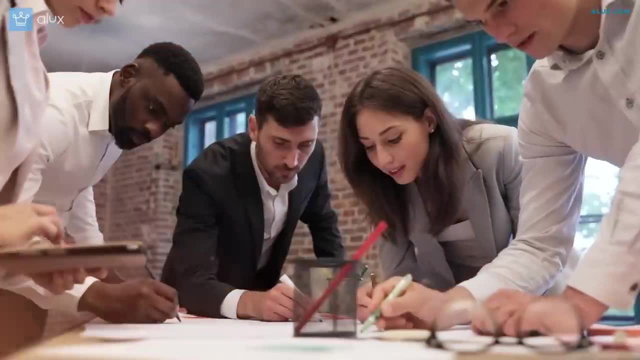 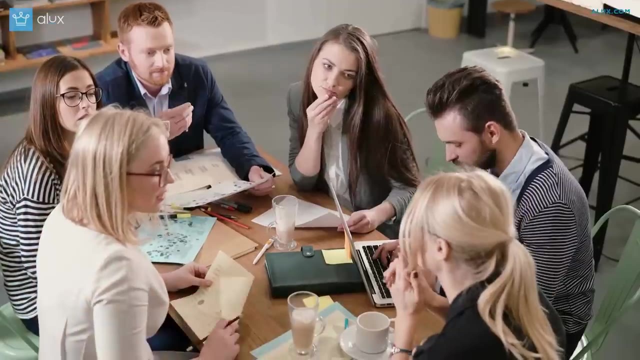 This strategic inclusion not only amplifies the richness of insights, but also catalyzes the emergence of innovative and comprehensive solutions. Moreover, collaborative efforts cultivate an environment where the boundaries of conventional thinking are pushed. Unified minds allow for the fusion of ideas that might otherwise remain isolated. 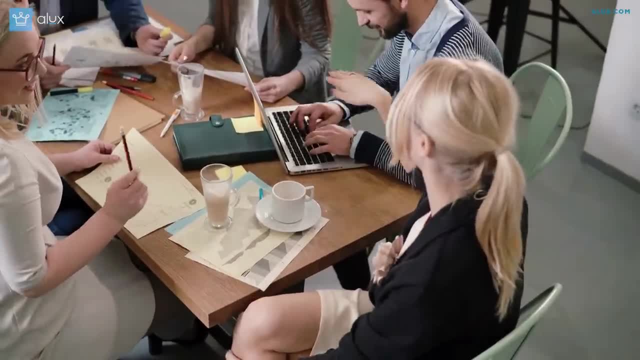 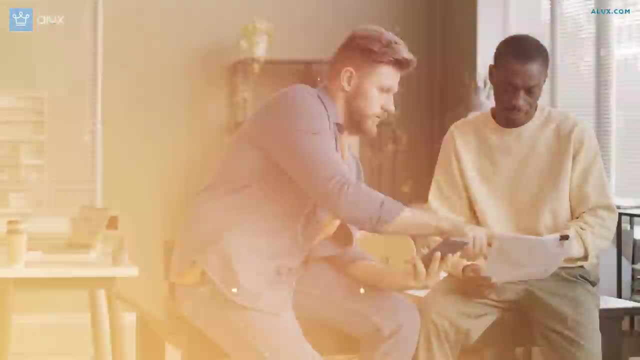 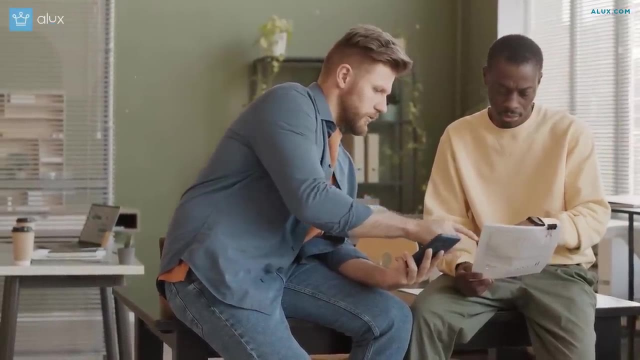 This fusion births solutions that are both transformative and pragmatic. By integrating diverse perspectives, you get to assess the potential of your solution and you get to a solution significantly quicker. This cooperative approach enhances your problem-solving arsenal, enabling you to not only overcome challenges, but also pioneer novel solutions that resonate with innovation and efficacy. 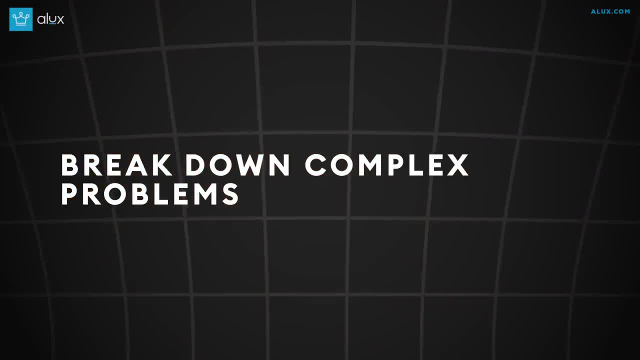 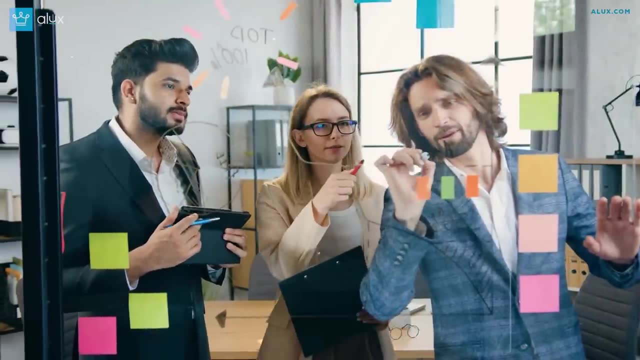 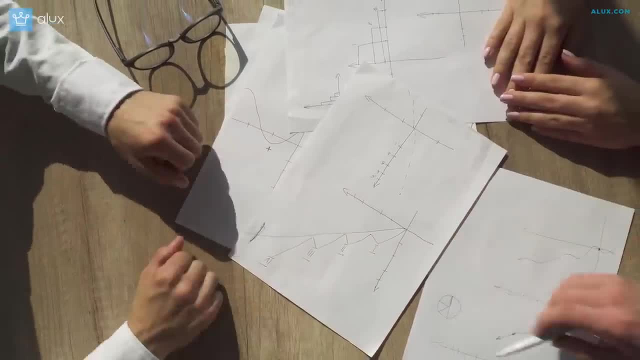 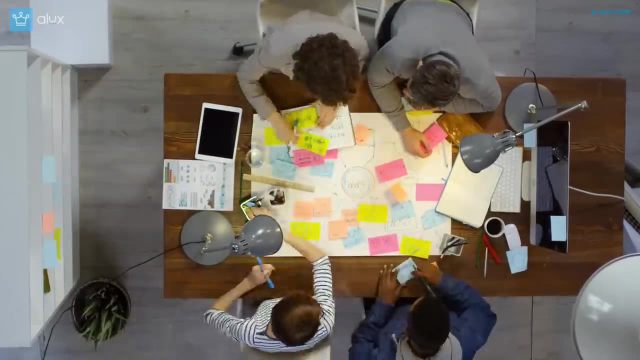 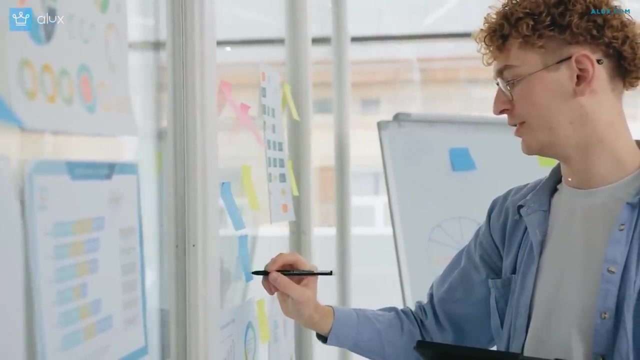 This involves breaking down the complex issue into smaller, more manageable challenges. By doing so, you're also able to navigate the labyrinth of complexity with clarity and finesse. Visualize this approach as disassembling a complex puzzle into its individual pieces. Each piece represents a distinct facet of the problem which can be addressed separately. 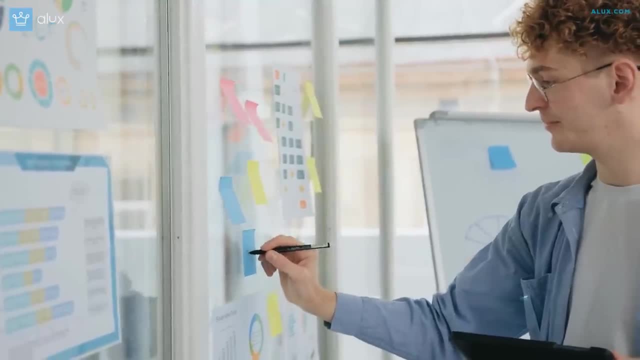 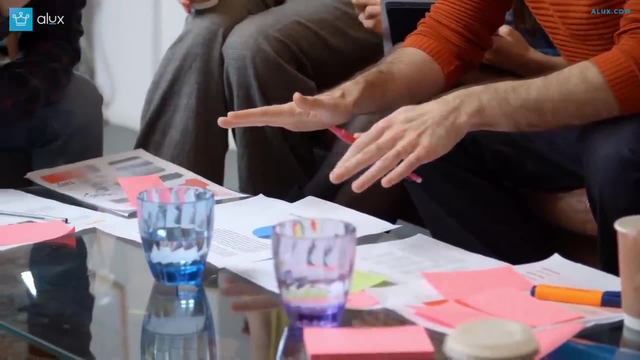 This dissection simplifies the challenge, allowing you to focus your energies on solving each component methodically. Methodical deconstruction and subsequent integration of the problem can be a key factor in solving the problem. Many solutions over time facilitate a well-orchestrated approach to complex challenges, which prevents 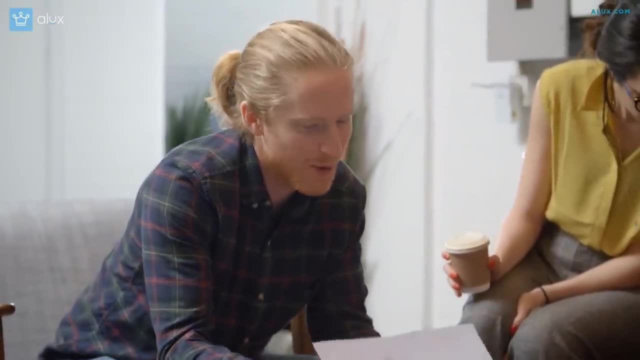 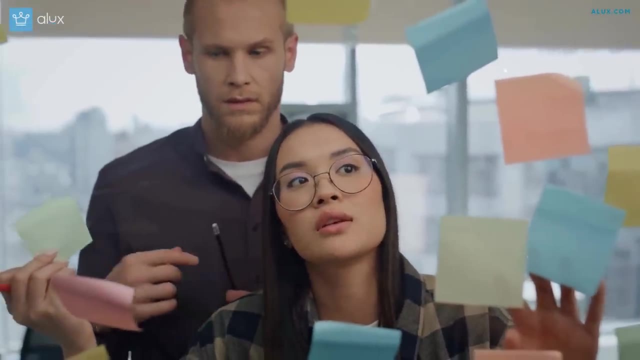 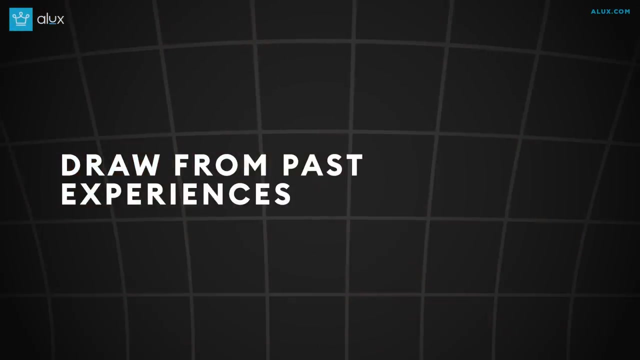 overwhelm, streamlines your efforts and enhances your problem-solving efficiency. This breakdown is the keystone that unlocks solutions to even the most complicated problems. Draw from past experiences. You need to draw upon your personal history as a reservoir of wisdom when confronted with present challenges. 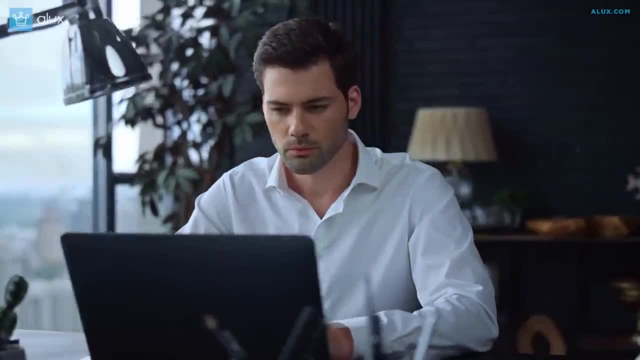 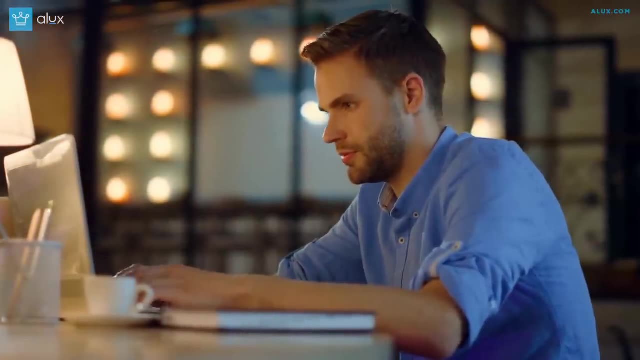 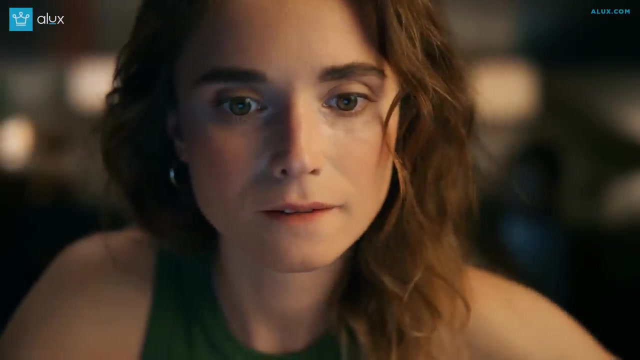 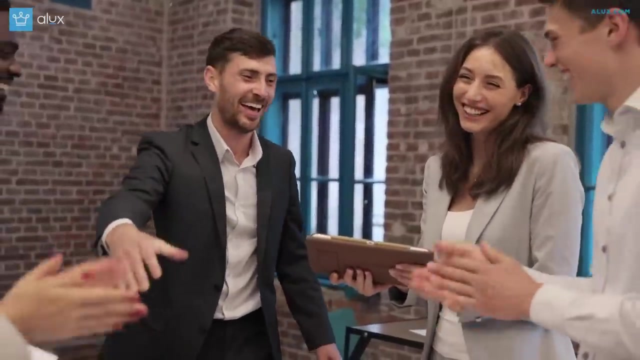 The journey you've traveled is rich with experiences, each chapter containing valuable lessons waiting to be wisely deployed. So imagine these experiences are stepping stones, Reflect on the past challenges that you've overcome, extracting the insights that are applicable to your current situation. Every obstacle you've conquered harbors a drop of wisdom, a key to unlocking solutions. 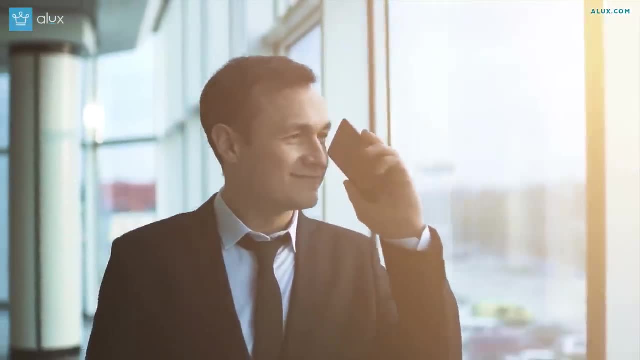 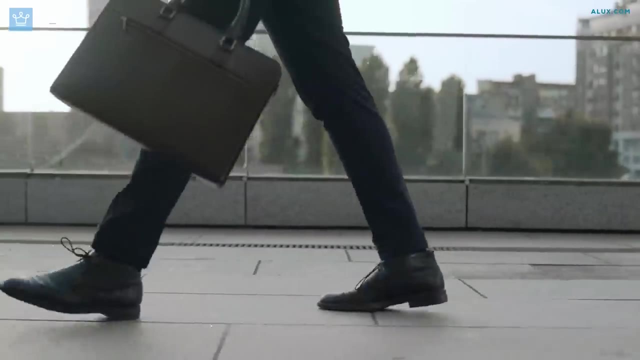 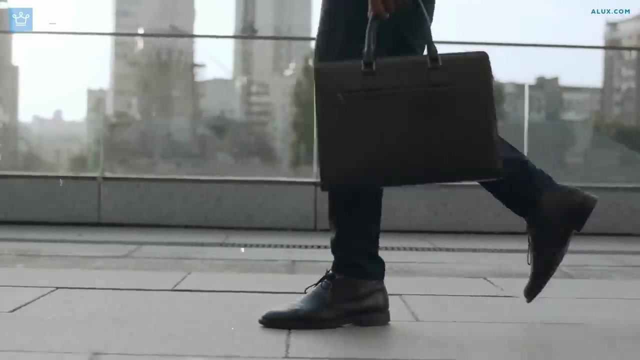 for the present. Incorporating the wisdom of your past into your present efforts transforms you into a dynamic problem solver. The pages of your history aren't just tales of the past. they're blueprints for the future, empowering you to conquer new challenges with a wealth of acquired knowledge and perseverance. 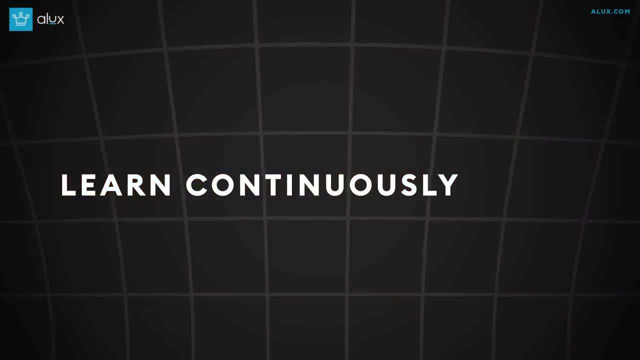 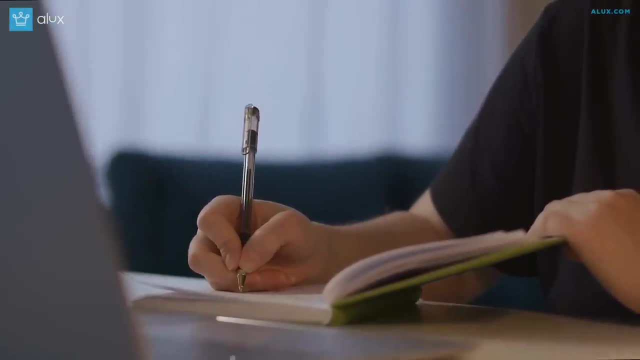 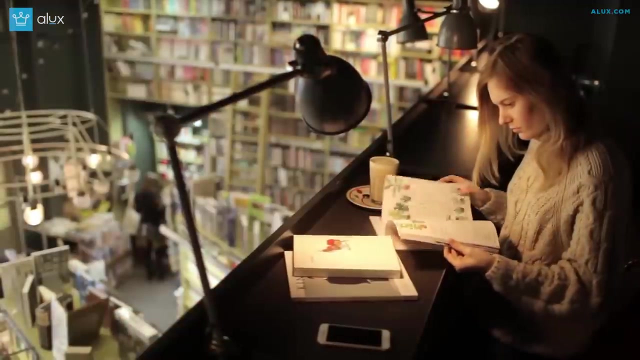 Learn Continuously. Embrace the infinite potential of continuous learning and skill augmentation. Just as a garden flourishes with care and nurturing, your problem-solving skills bloom with the infusion of knowledge and expertise. Envision your knowledge and skills as the building blocks of your problem-solving toolkit. 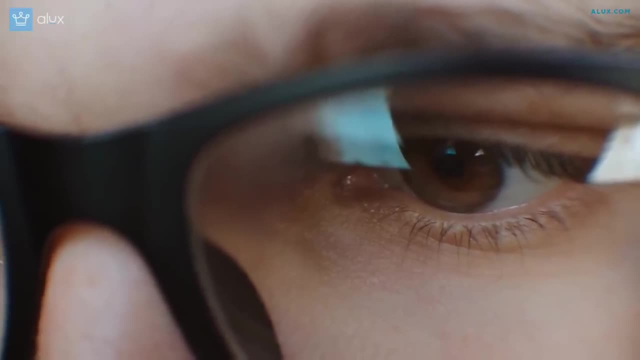 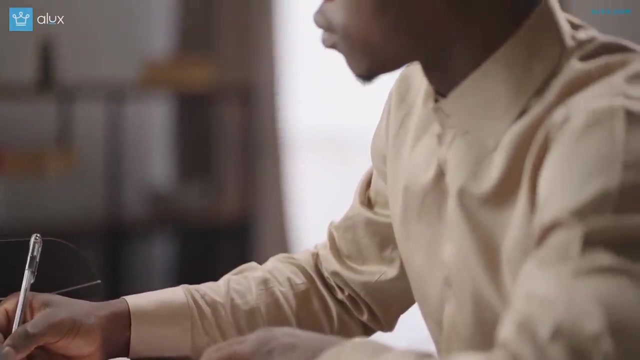 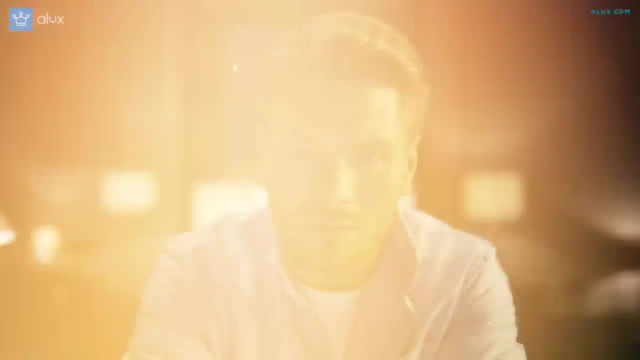 Try it, Try it. Welcome to the invaluable lessons that failures can impart. Each endeavor, even if it doesn't yield the desired outcome, is a step forward. This attitude dismantles the notion of failure as a roadblock and transforms it into a catalyst. 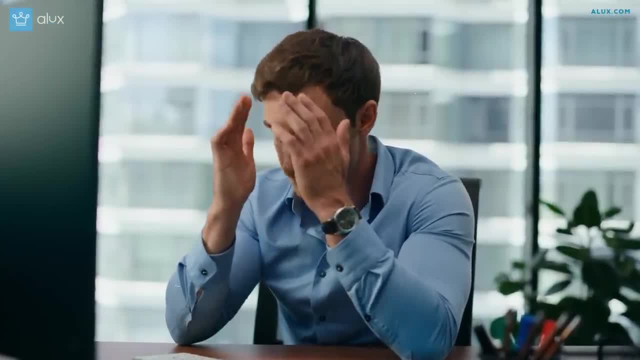 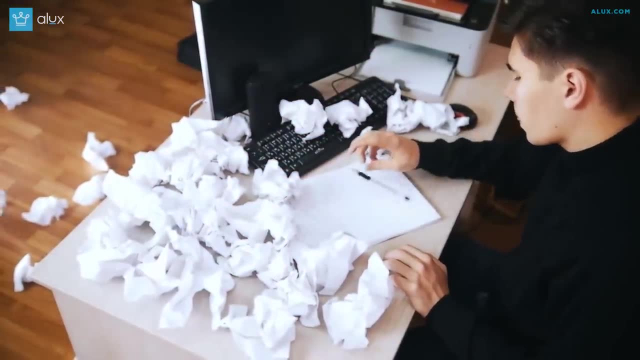 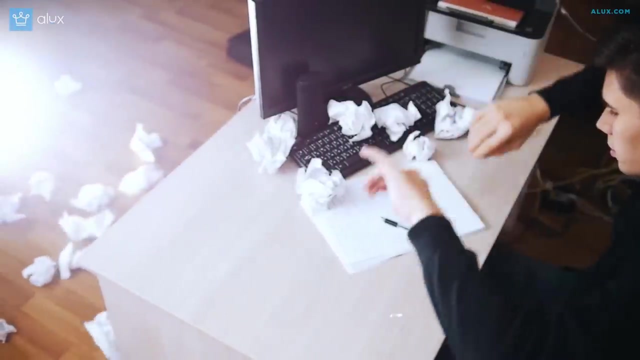 for growth. In this dynamic landscape of trial and error, each misstep is a potential springboard for innovation. Failure's lessons equip you with the wisdom to adapt, pivot and evolve- And evolve your strategies. The essence of this approach lies in its resilience. 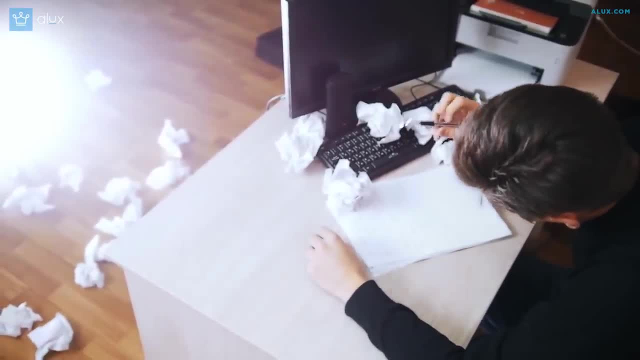 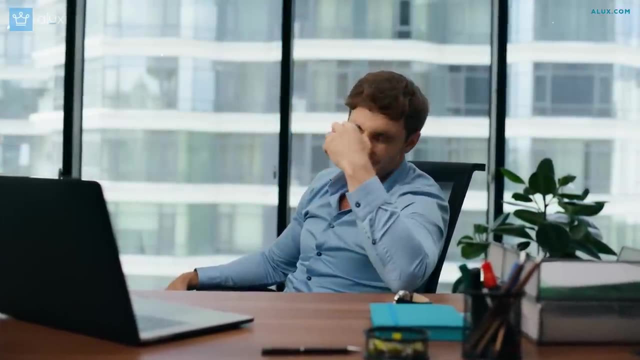 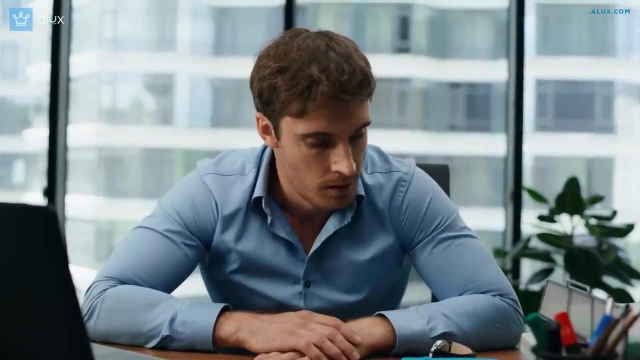 By removing the fear of failure, you empower yourself to venture into uncharted territory. This fearless mindset allows you to learn from every experience, whether it culminates in success or not, ultimately guiding you toward more refined and effective approaches. 3. 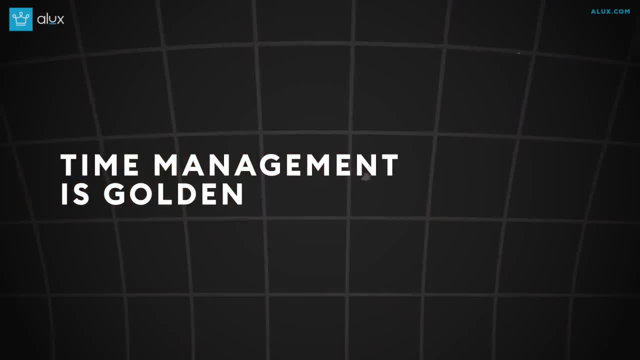 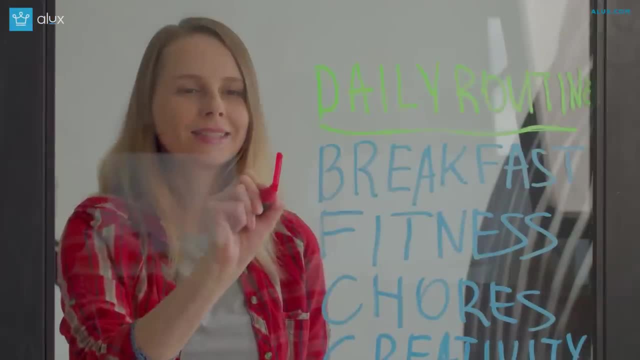 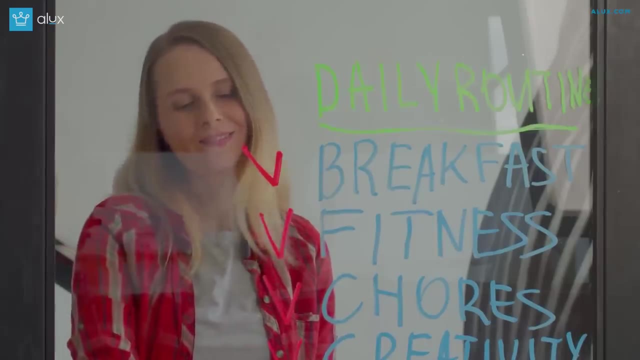 Time management is golden. 4. Immerse yourself in the art of problem solving by allocating dedicated time to a specific issue. Just as an artist requires a canvas and focus time to craft a masterpiece, problem solving demands a sanctuary of thought and contemplation. 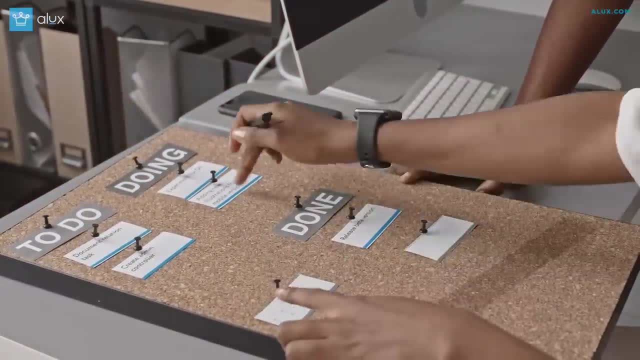 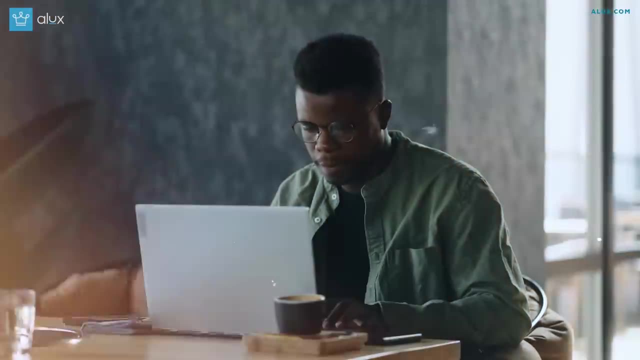 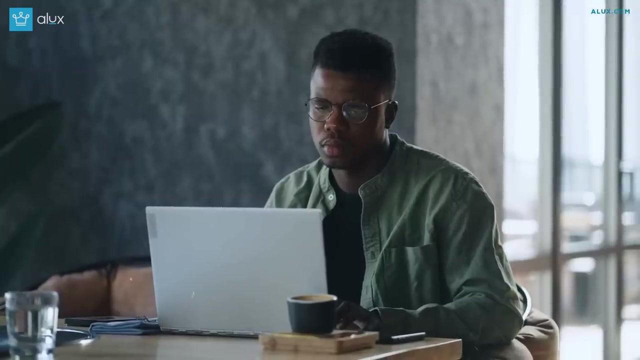 Resist the temptation to rush through the process. Much like a delicate symphony, problem solving thrives in the realm of patience and depth. 5. Give yourself the luxury of time to delve deeply into the challenge, understanding its intricacies and potential implications. 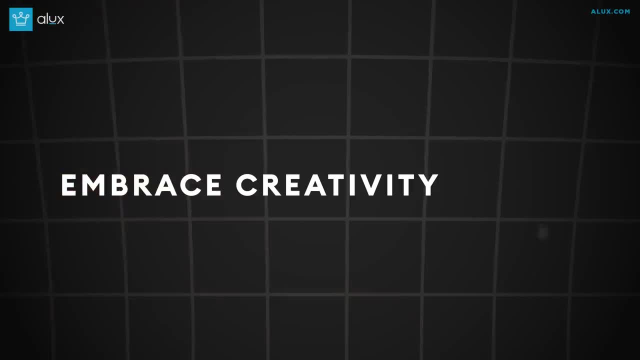 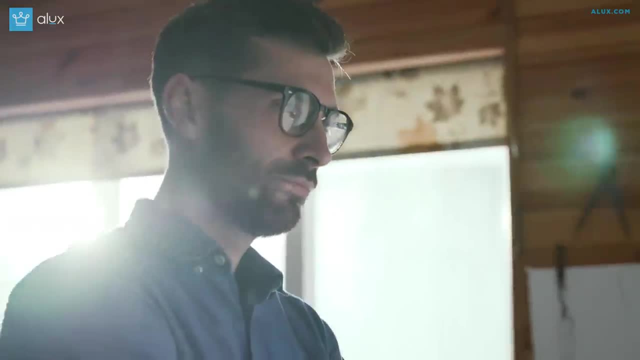 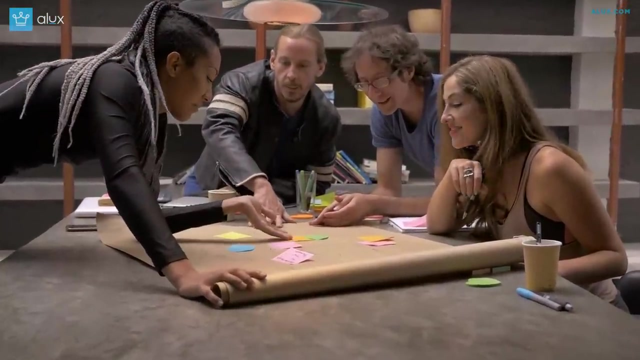 6. Embrace creativity. To truly think outside the box is to transcend the limitations of routine. Picture your mind as an explorer charting uncharted waters. In this mental expedition, allow yourself to entertain unconventional solutions that might initially appear far-fetched. 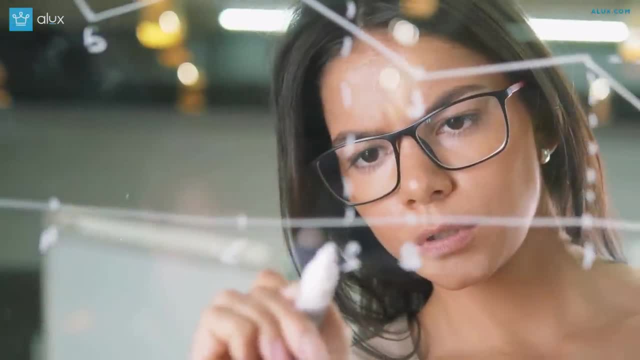 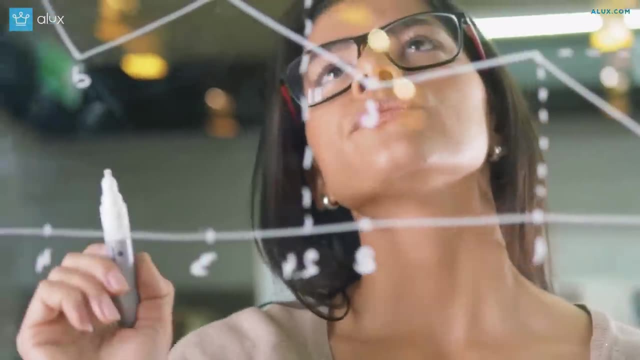 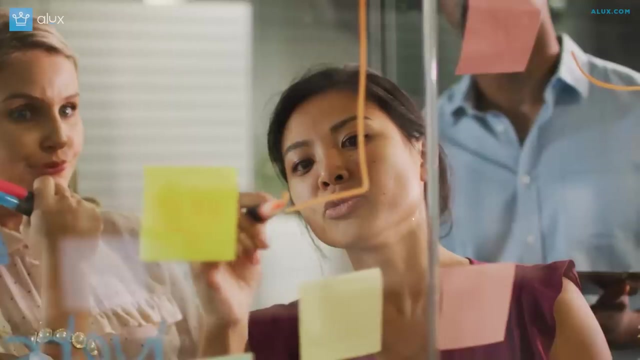 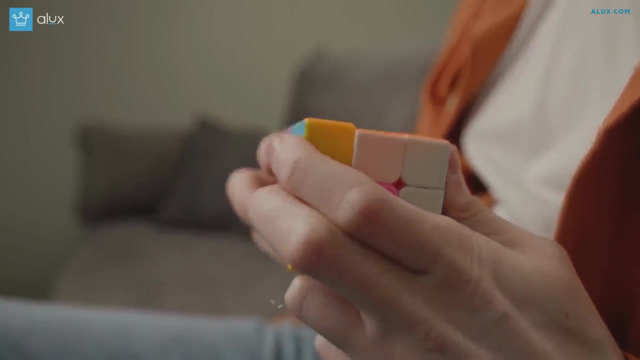 7. The beauty of this approach lies in its potential to unlock breakthroughs. Conventional methods often follow crowded paths, while creativity forges its own new trail. By embracing novel ideas, you uncover hidden opportunities that traditional avenues might entirely overlook. So, in essence, by opening the doors to creativity, you open the doors to breakthroughs. 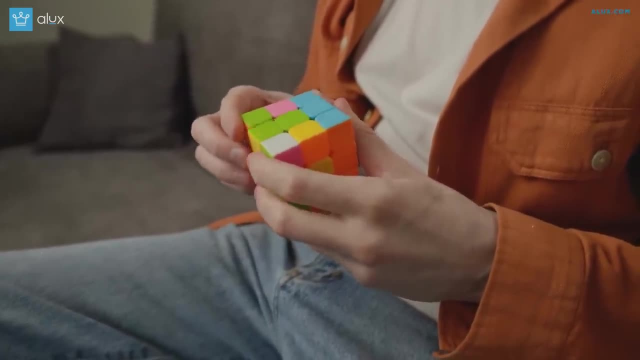 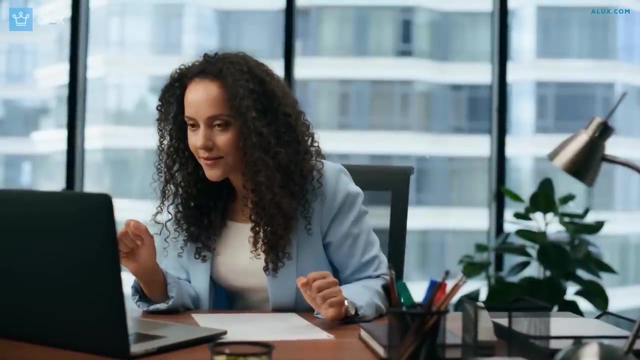 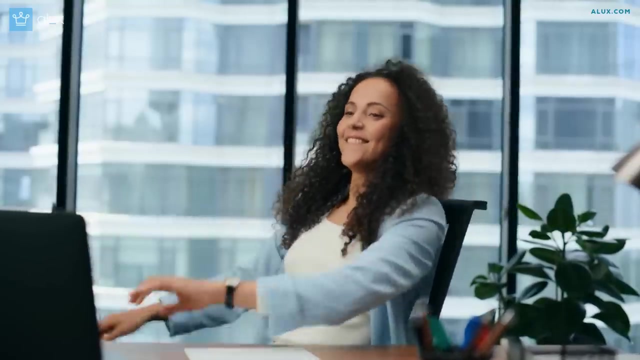 Creative problem solving is the compass that steers you toward solutions that will help you challenge the ordinary and illuminate the extraordinary. It's in this expansive realm that the seeds of innovation germinate, sprouting into solutions that resonate with ingenuity and effectiveness. But you've got to learn to stay calm under pressure. 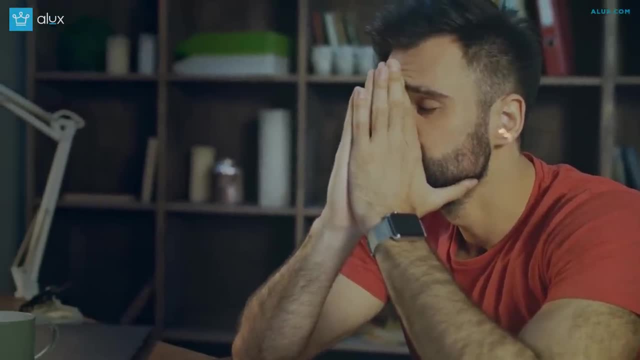 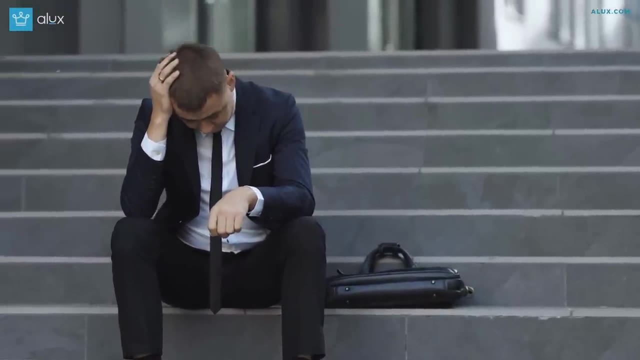 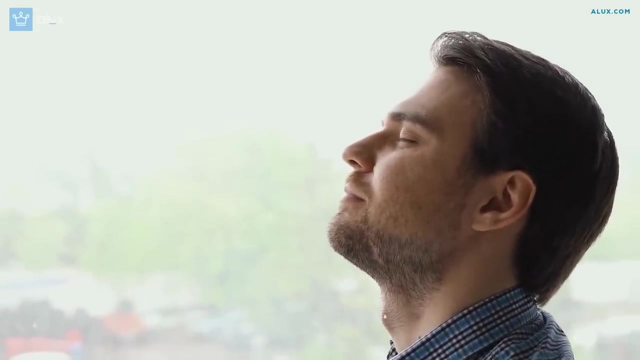 Recognize the profound impact of pressure and stress on the landscape of problem solving. These adversaries have the potential to cloud your judgment and impede clear thinking. However, you possess the tools that can act as shields against their influence, enabling you to navigate the tumultuous waters of high-pressure situations with composure. 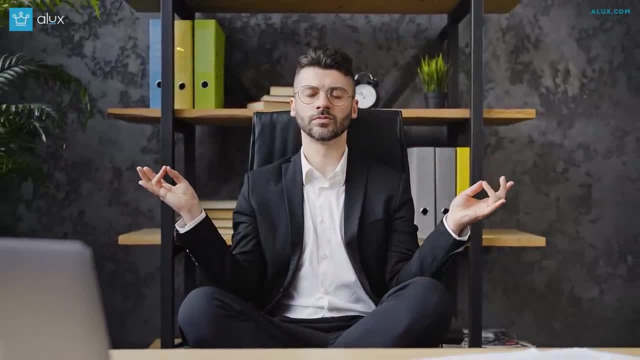 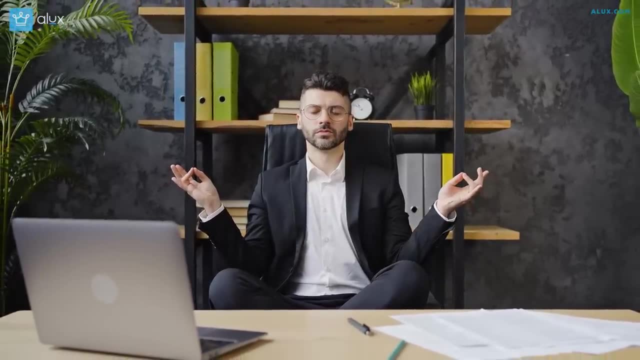 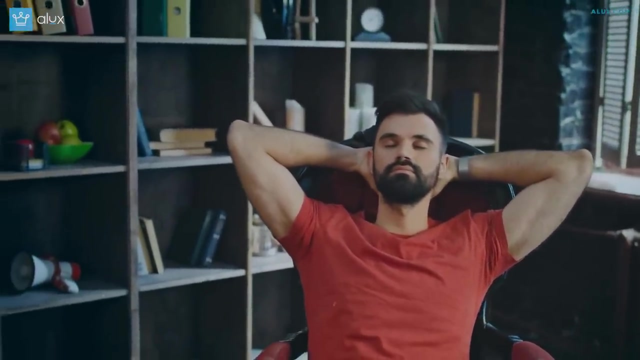 Imagine these tools as a sanctuary of calm within the storm. Techniques such as deep breathing and mindfulness are your anchors, grounding you amidst the chaos. Deep breathing provides a lifeline, infusing your system with oxygen and tranquility, dissipating the fog of stress. 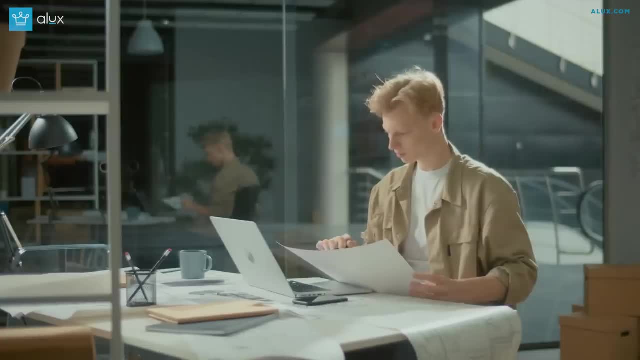 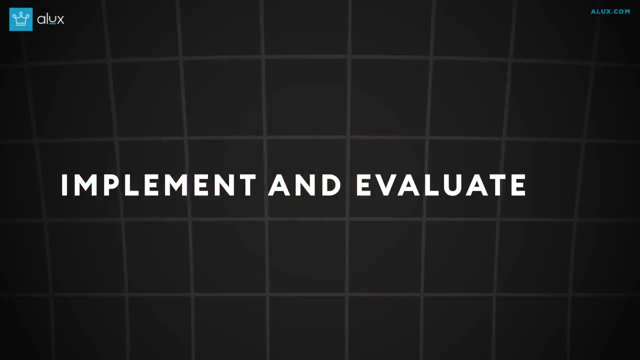 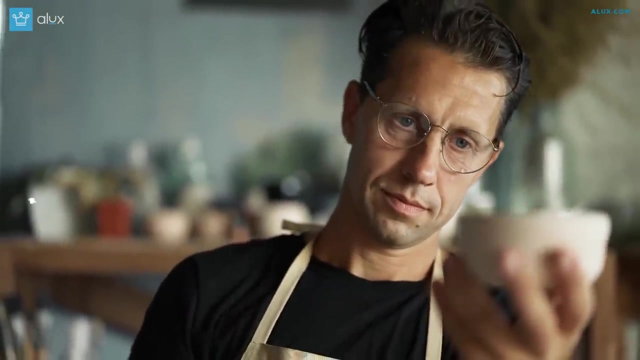 Mindfulness, on the other hand, cultivates a focused awareness of the present moment, preventing stress from totally hijacking your mental resources. And lastly, of course, you need to implement and evaluate. The culmination of your problem-solving journey lies in the implementation of your chosen. 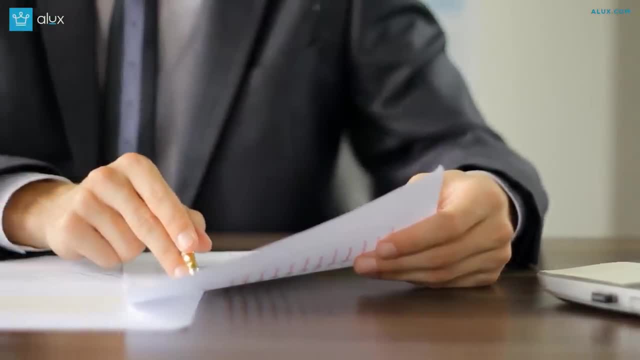 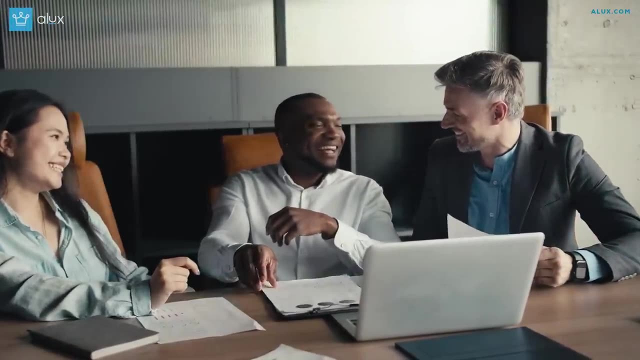 solution. This phase is a voyage into action, where theory transforms into reality. As you navigate this terrain, remember that the journey doesn't end here. The journey will continue. It doesn't end with implementation. It extends into the realm of vigilant observation and adaptive refinement.